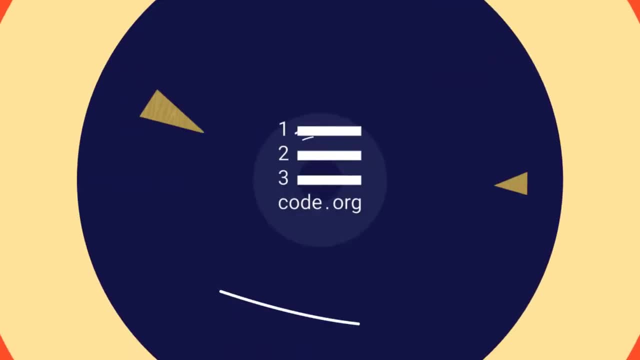 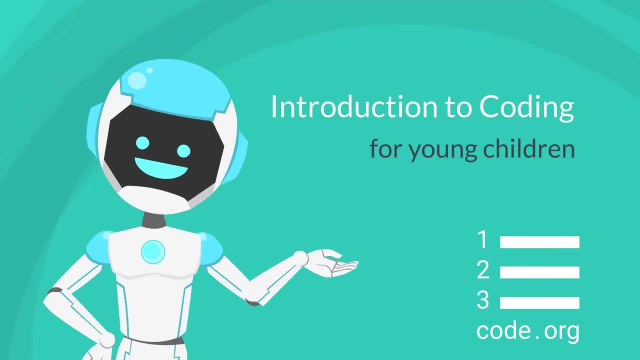 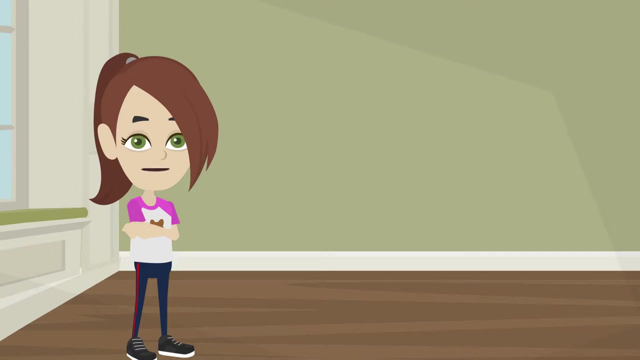 Hi, I'm Evie and I want to tell you all about coding. This is my robot. I call her Cody because I can give her instructions and she follows them. Cody, wave your hand Now, clap your hands for three seconds and do a little dance. 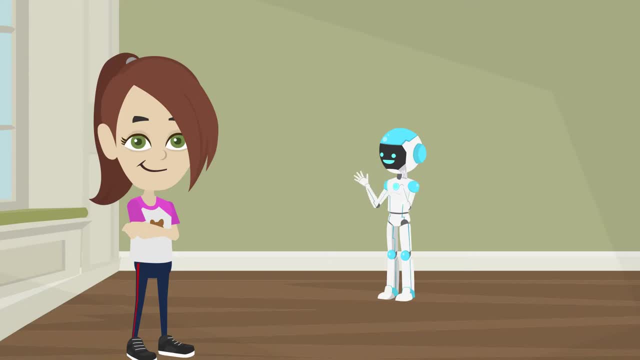 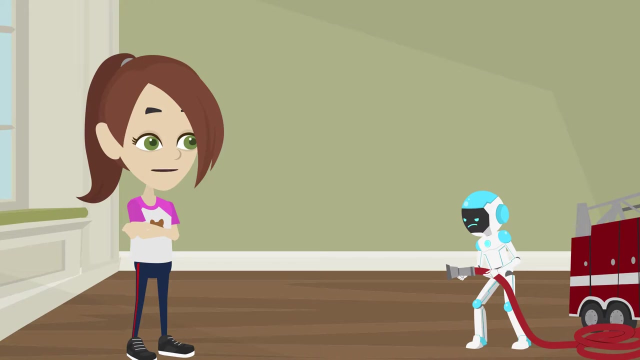 Cody has a computer inside her that knows how to follow my instructions. Cody, please go and get me a drink. I'm not that thirsty. Cody, when we give instructions to a computer, we need to tell it exactly what we want it to do. Otherwise it mightn't do what we want. 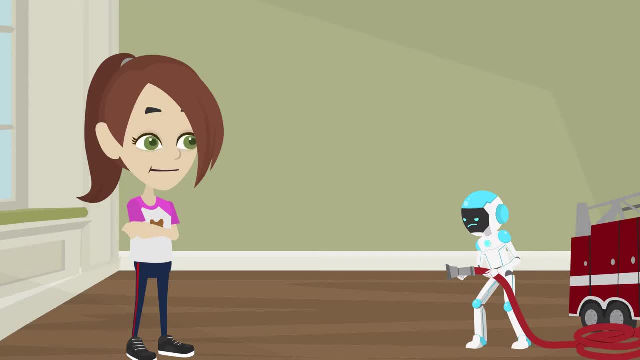 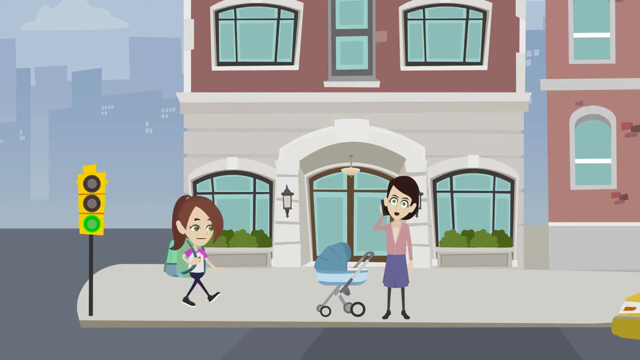 Cody, can I have a glass with water in it please? Thanks, Cody, that's better, Right, we better get to school. Lots of different things have computers in them. Cody, can you give me a drink? every uniform has computers in them: Phones, airplanes and even traffic lights. 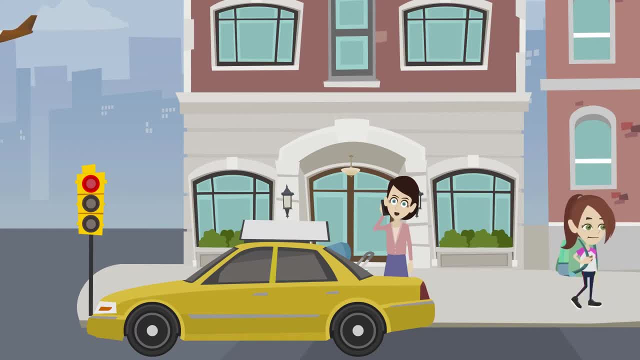 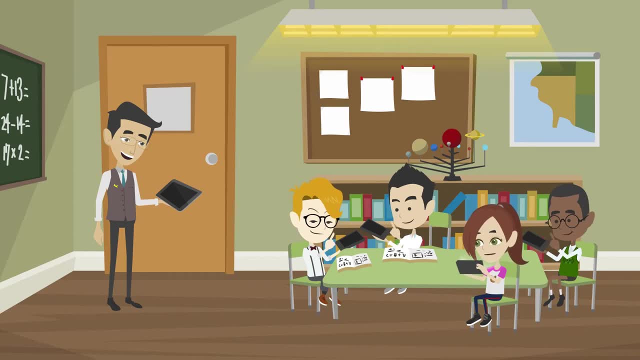 have computers inside them. When you are giving a computer some instructions, it's very important to put the instructions in the right order. Okay, class, I want you to look at your tablets and try and put these steps in the right order. If you were putting on your shoes in the morning, what order? 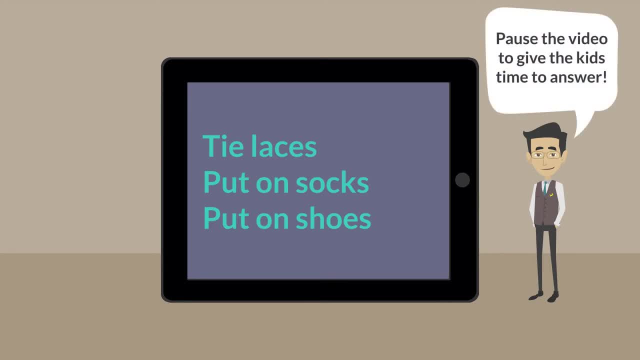 would you do these steps in? The correct order is: 1. Put on socks. 2. Put on shoes. 3. Tie laces. If you were brushing your teat in the morning, what order would you do these in?